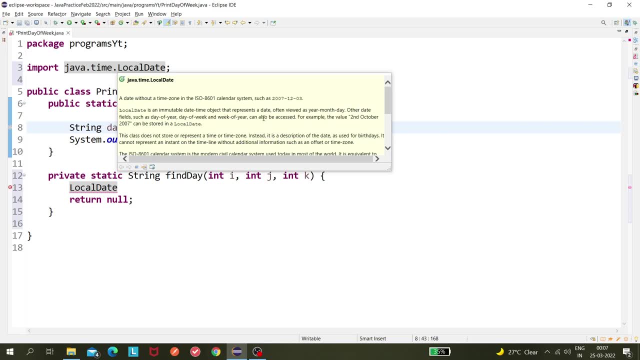 such as day of the year, day of the week and week of the year can be also accessed. so we need like day of the week, so we need this one and next. for example, the value of second October 2007 can be stored in local date. okay, so this is a huge. I mean lots of methods would be. 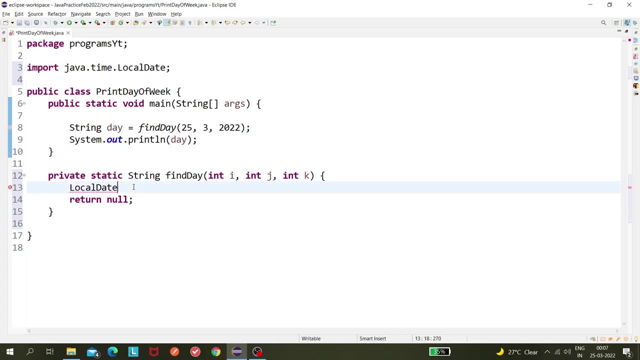 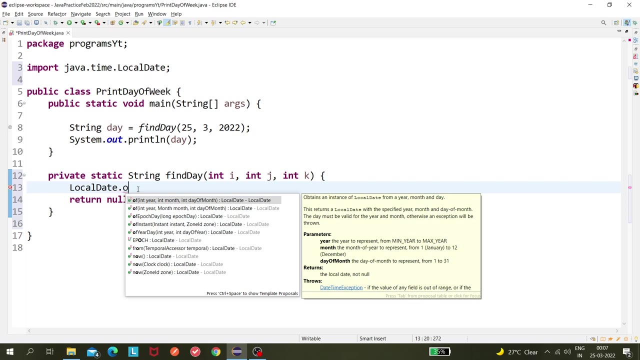 there. so let's see how can I utilize all that's that thing here with the help of local date class. so okay, so local date dot. there is a method code off so you can see this of method. this return a local date with specific year, month and. 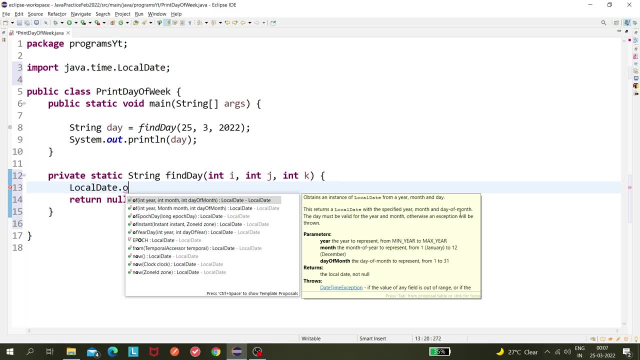 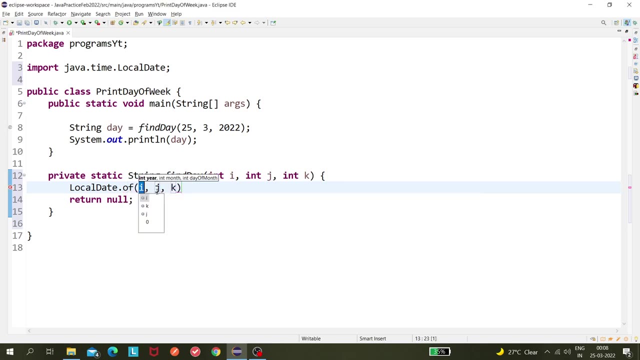 day of the month. so day of the month means it is also integer. so that means in here we need to pass this. here: value 20: goin integer month. we need to pass three. integer day of the month, month: we need to pass 25. so let's take it and here I will be writing: is I? 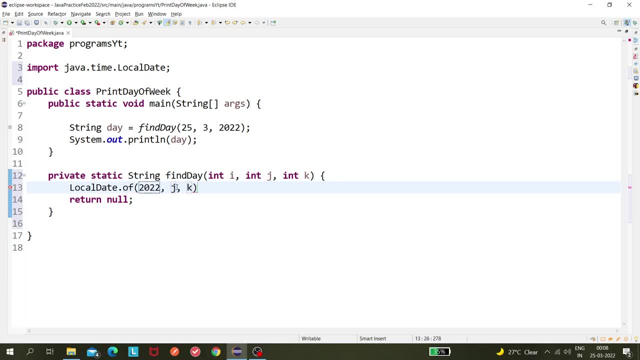 instead of I will be passing it as 2022, and then here I will be passing three and here I will be passing 25 semicolon. so this will be returned something right? so we do not know what we know already. it will be returning local date, but 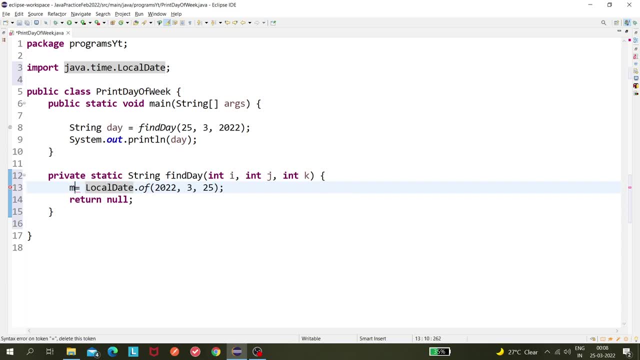 still, I am just writing like my date and sorry, my date, and here I'm overing over it. so it's literally saying that: create a local variable. I am clicking on it and you can see it. this eclipse, or eclipse has eclipse- helps us to you create this local date. so even though, if you do not know, with this help of eclipse, 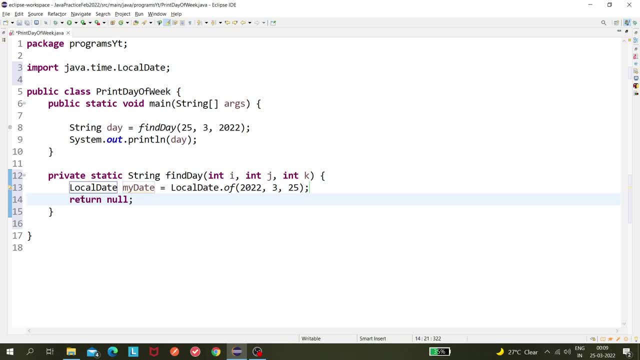 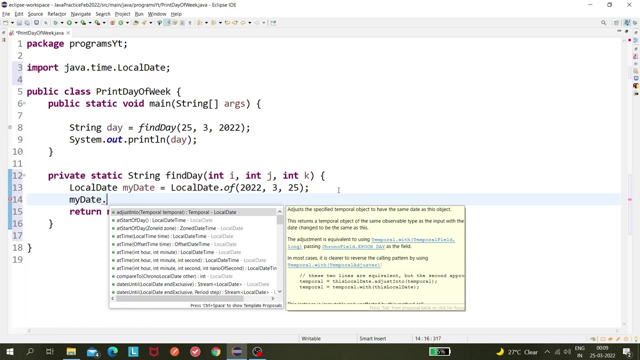 we can create, you can get it right, okay, okay. so next I'll be moving to my date. so now my date. object: dot. and let's say: if you have, if we have, any methods which can be used to find the day of the month, so day of the month, get day of month. or get day of week right, so get day of the week. so 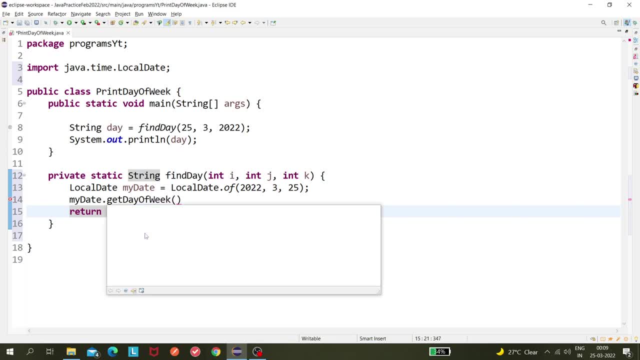 let over. let's over over it and see what it is returning. so gets the day of week field, which is an enum day of the week. so this method returns the enum day of the week. so if I click on it, so a day of the week, such as Tuesday. okay, so this day of the week is a enum and it is. 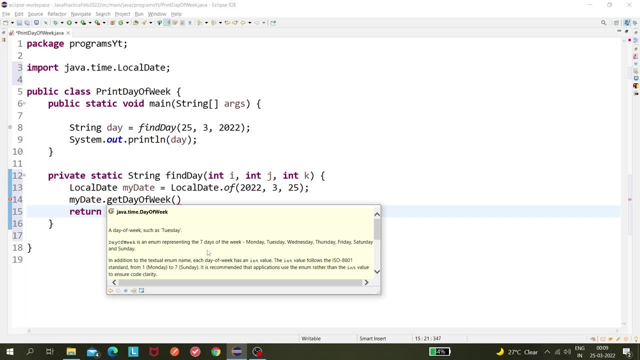 having. it is actually an enum representing seven days of the week, like monday, tuesday, wednesday, something like that, till sunday. so monday is the first and sunday is the last day of that week and in addition to that extra term so you can read about it and so basically this get day of the week is returning the enum, which is day of the. 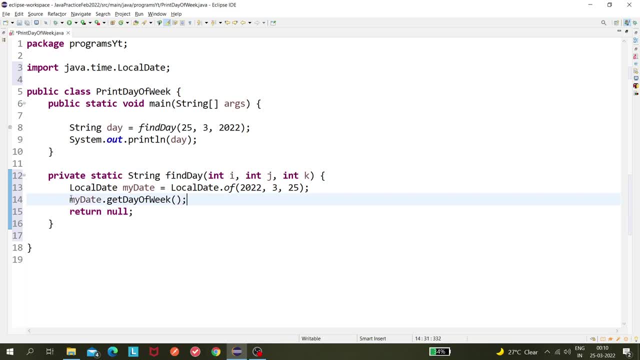 week, okay, so i'm just putting semicolon and here i'm writing day of the day of the week. so this is my variable, which i'm creating, and it is actually returning in the enum. so i'm just over writing here local variable, so which is day of the week. so we got the 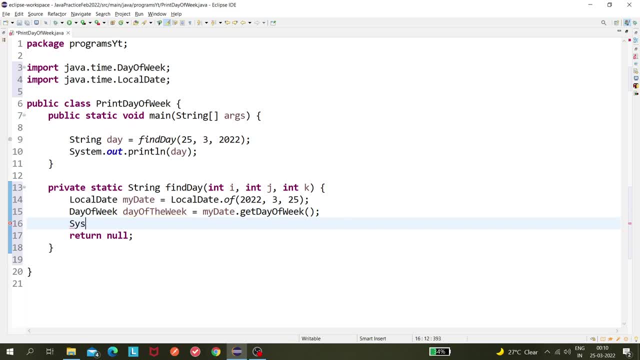 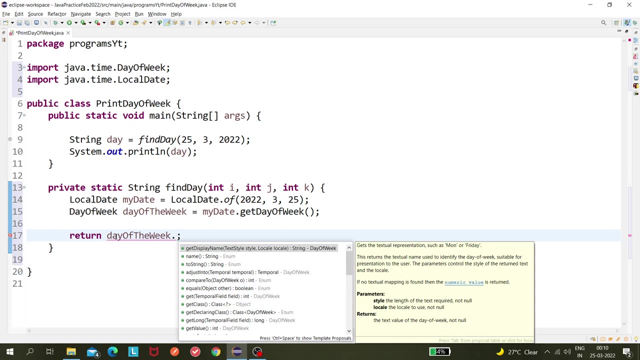 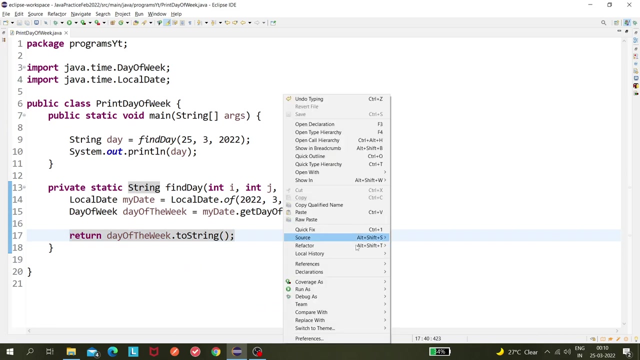 day of the week. now i will print sysout, okay, or maybe we can write like return day of the week, dot dot dot to string. yep, yeah, so let's run it and see what it is printing. so it's printing friday, absolutely right. so our program is currently working and let's change it to something in past probably. 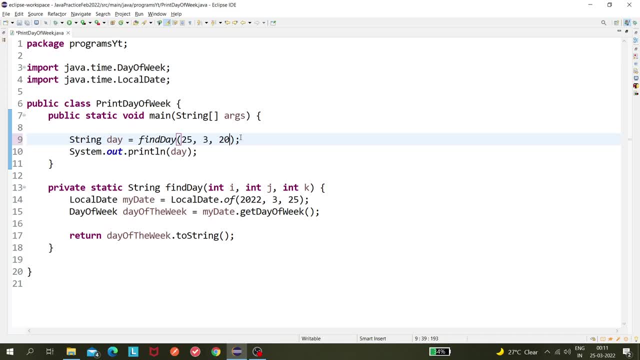 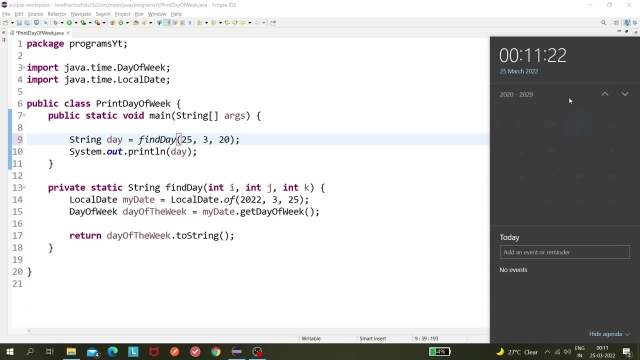 we can check. for example, lets go back to the calendar and check here. so click on here. so i'm going back over here, so it will be just summer. so, friends called out here, that's all for today and i think this work is big and fun. so if you guys like this video, you will like it later. if you guys will give me recommend some tests, then i can give you daily express けっ Stacy at my website address in the description. so let's go back to your that and so looks. see the initial program transfer procedure. if you don't wish to take any option, see result. 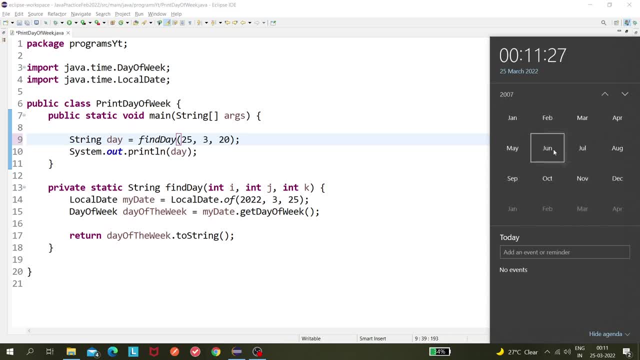 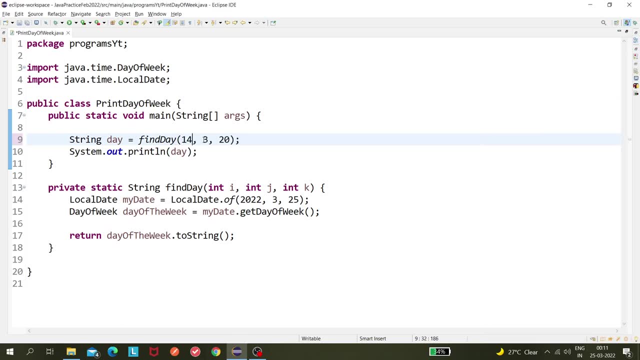 if you guys like this video, this arm configuration. so when someone um- and i'm going to again run old file delivery which me set a certain sieve, and or they fill the random photos from shutting up to 2007 and June month and at 14th, so 14 June 2017, so let's do that: 14 June 2007. 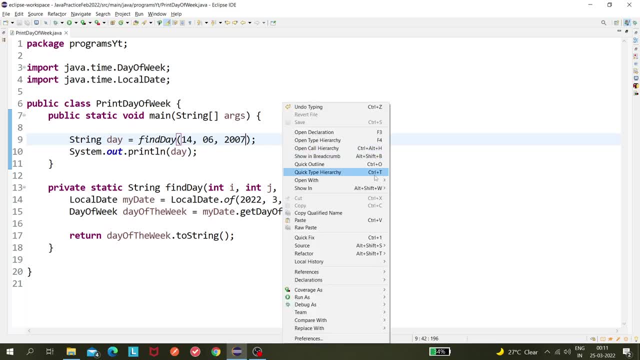 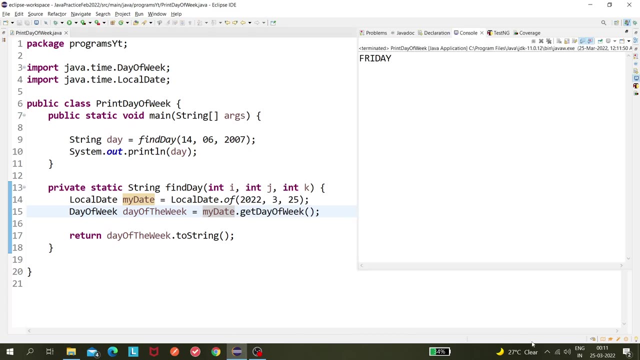 7, so it was, I think, right witness day, believe. okay, probably it is not saved, or I did a mistake. okay, it is returning again. oh, okay, sorry, I mean I did a mistake, right, because I'm just hard-coded it here, right, so that's the wrong thing. so where we have to do integer year, integer month and integer, 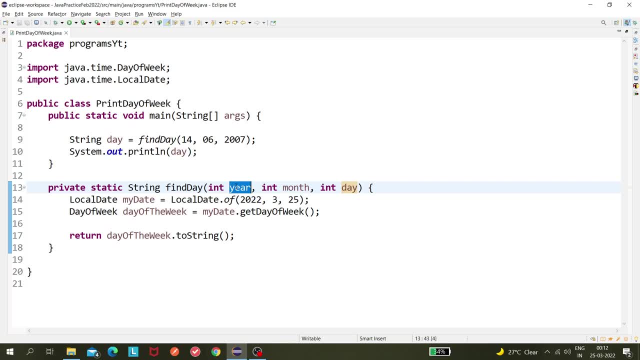 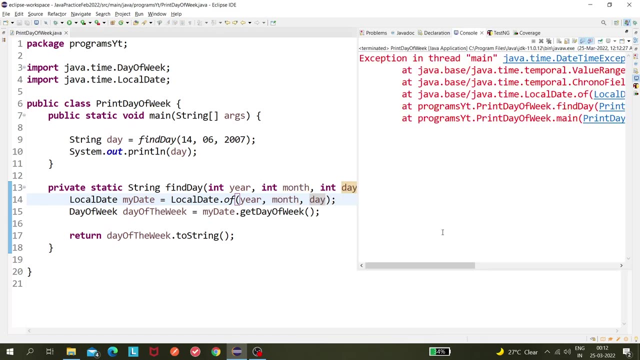 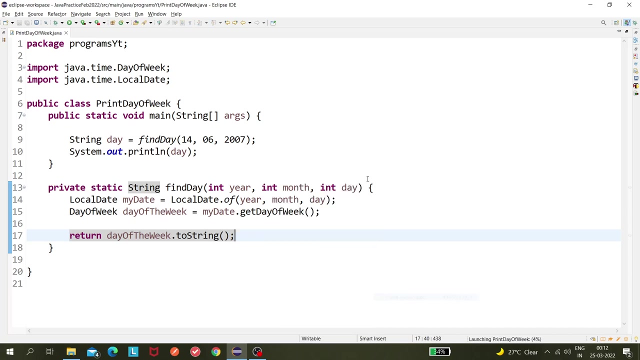 day, so here we'll be going here and month would be coming here. this is the day, so if I run it now, I hope okay, it's giving some error right. so let's see what is the error. it's giving, sorry, invalid value of day of the month valid 1 to 28. 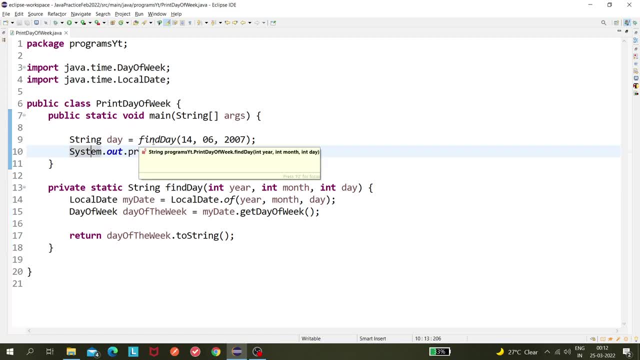 okay, so Friday internet yet okay, sorry, sorry, I didn't mistake here again. so this is 2007 and find it and this is month, so find days, actually having into your your month and day. so this is would be handlar day and di textbook and yiliah. it is every day, so I'm not going to change it. 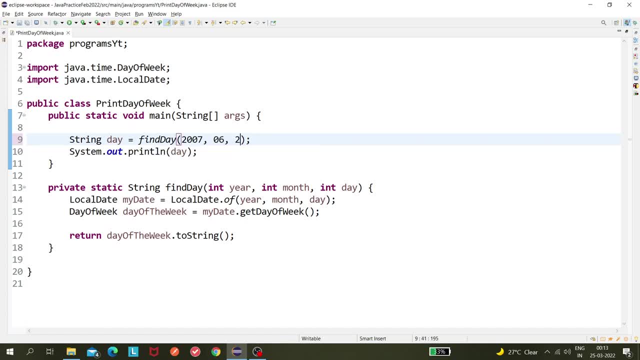 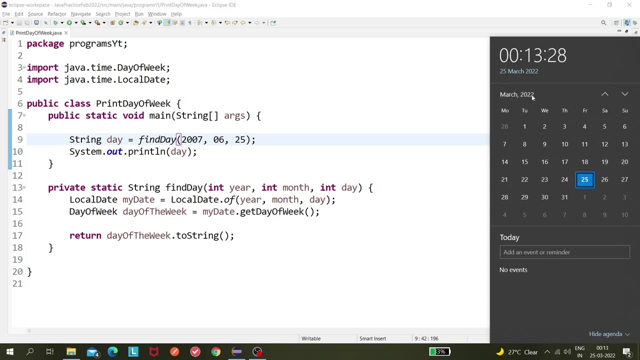 so find means actually having into a year, month and day. so this is what we would be: 25th, right, and it's actually check. it go back to 2022, 2007, 2008, June, and I'm checking 25th of June, so it should be Wednesday, so 2008, and now run it. 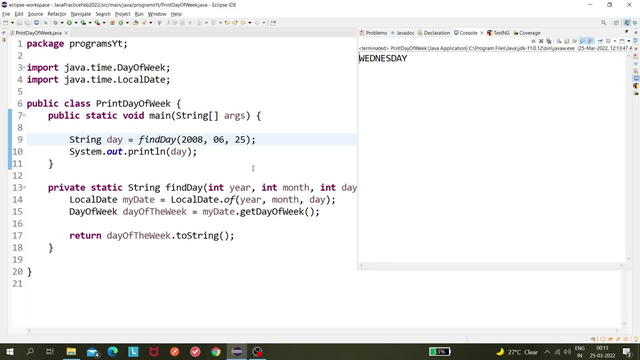 yep, so it's working fine. so like this, we can get any day of the week from any particular date. I hope you have understood it. thank you for watching.